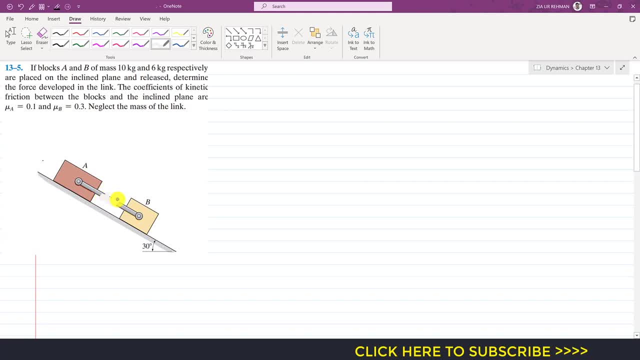 consider the free body diagrams of block A and block B separately and we will analyze both the blocks one by one. So now, as we can see that the weight of this block A will be acting vertically downward and it will be 10 times 9.81.. So 10 times 9.81 is 98.1 newtons and similarly, this inclined plane will apply the. 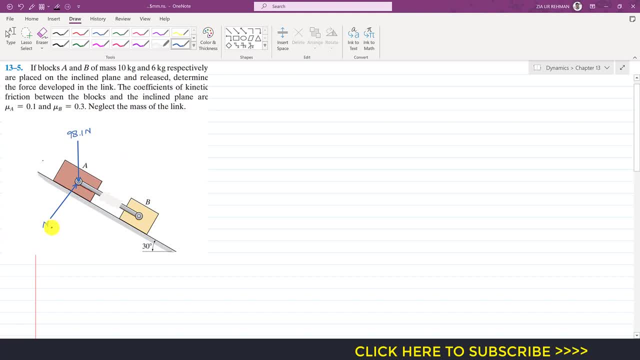 normal force on this block A, and let's say that is represented by N A, and as we know that if the inclined plane is making 30 degree with the horizontal, then this weight will be making 30 degree with the horizontal. So we can resolve this weight into its components. So it will have two components, One of its 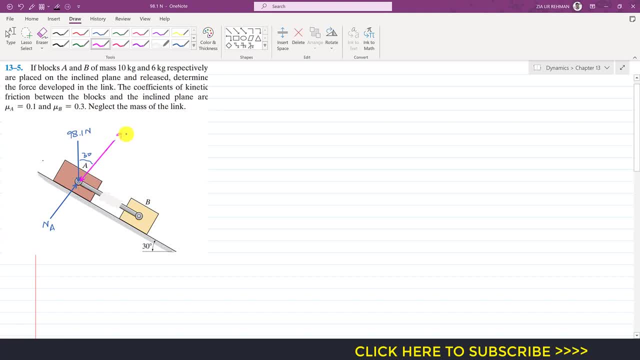 component will be acting like this: This one will be the cos component. We can write this: 98.1 cos of 30 degrees, and similarly we will have one another component like this. This one will be the sine component. This is 98.1 sine of 30 degrees, and similarly we will have 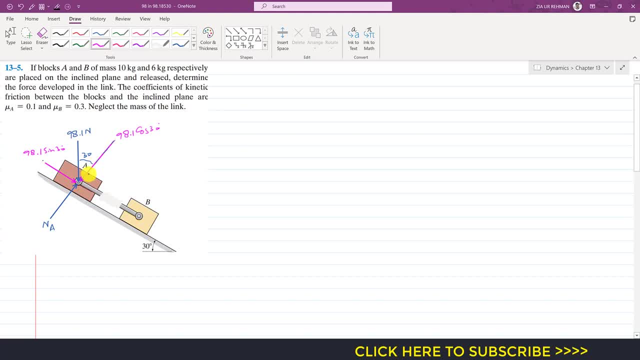 one, R N, as we can see over here. So this one is watching flat and keep doing the same work here To find out. R? N is various modes of attraction. So what means R is that there is a force which is brought in the opposite direction- the plane- but it is there motion. designed in the opposite directionands similarly, this block will apply the force on this block B with the help of this link. As a reaction, this block B will apply the force on this block A in the opposite direction. right, So we will have force in this direction. Let's say that this is that force which is developed in the length. So we are required to find this force. F. Now, if I come here and let's say I will have the force in front, we will find this precise force, prefered force. If I'm going in this direction, then this: 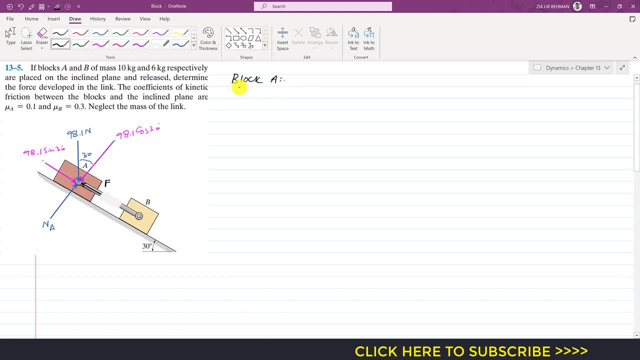 Consider block A and if I apply the equation of motions, if I apply the summation of forces along y equals to m, a, y and this is my positive x and y direction. right. Positive x is parallel to the inclined plane and positive y is perpendicular to the inclined plane right. 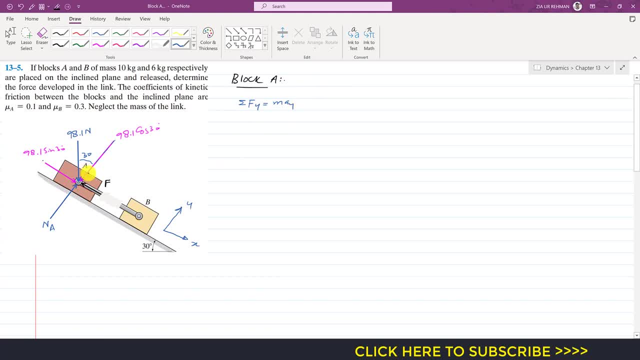 So now, as we can see that this n a is acting in the positive y direction and this cos component of the weight is acting in the negative y direction, So I have to write: this is 98.1 cos of 30 degrees and this will be equal to mass of block A right. This will be m a right, So m a is 98.1.. 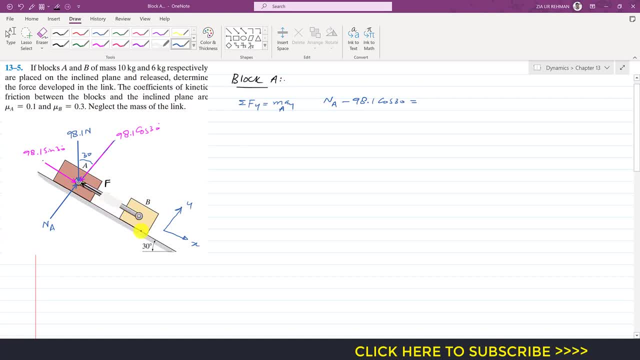 But as we can see that the blocks are only moving in the along the inclined plane right, So there is no motion along the y axis. So this means that the acceleration along the y axis is zero. So this means that m? a into a y will be equal to zero right. So now from this we can say that n? a equals to 98.1 cos of 30 degrees right. And similarly, as we know that there is a friction between the surface, between the two surfaces right, 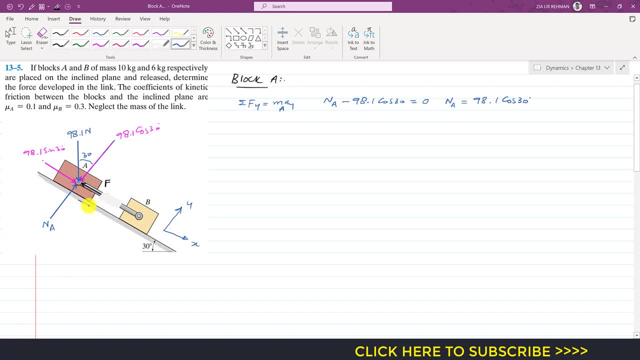 So if the blocks are moving downward, then what will happen is that the friction force will be acting in the upward direction and the coefficient of kinetic friction between the surfaces of block A and the inclined plane is 0.1.. So this friction force will be equal to 0.1 times n a right. So now, if we apply the summation of forces along x equals to m a a x right. So this is my negative x. 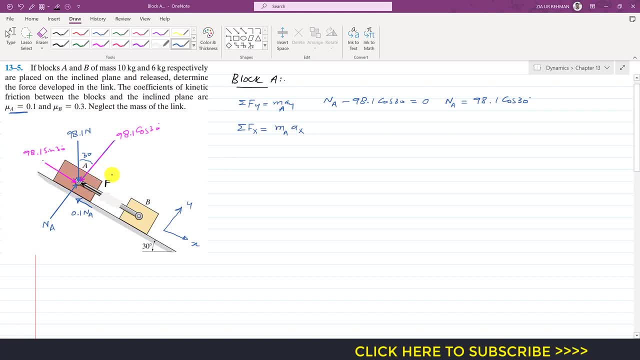 as we can see that this F is acting in the negative X direction, so I have to write minus F. this sine component is acting in the positive X, so I have to write plus 98.1, sine of 30 degrees. and similarly, and this friction force is acting in the negative X direction, so I have to write: 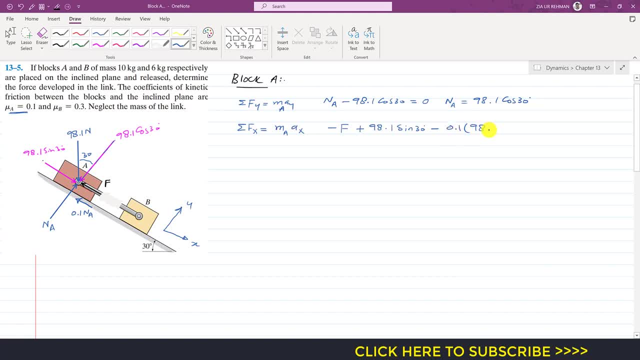 minus 0.1 and A, and then A is 98.1 cos of 30 degrees, and this will be equal to the mass of A, and the mass of A is 10 kg, right? so I have to write 10 and AX. so now we can simplify this. 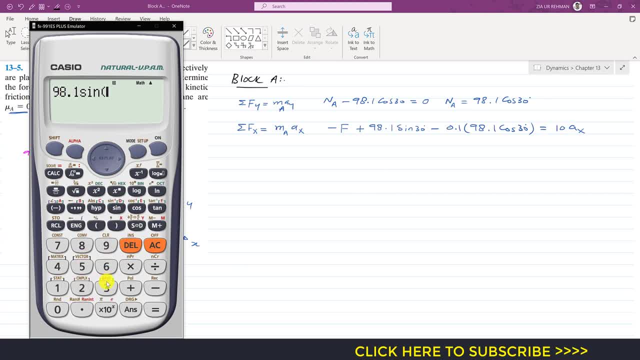 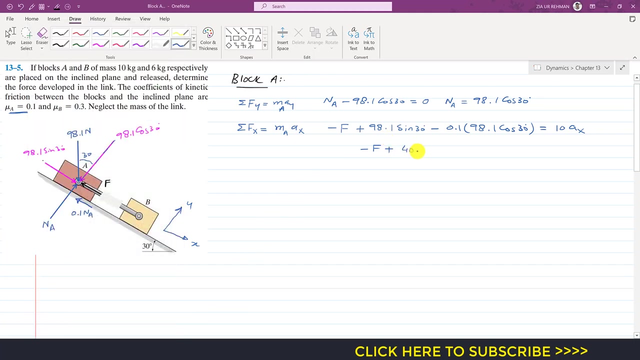 98.1 sine of 30 minus 0.1 into 98.1 cos of 30. so this is minus f plus 40.55. 40.55 equals to 10 ax, right. so now this is equation one. we have one equation and two unknowns. this means that we have to consider this block b. 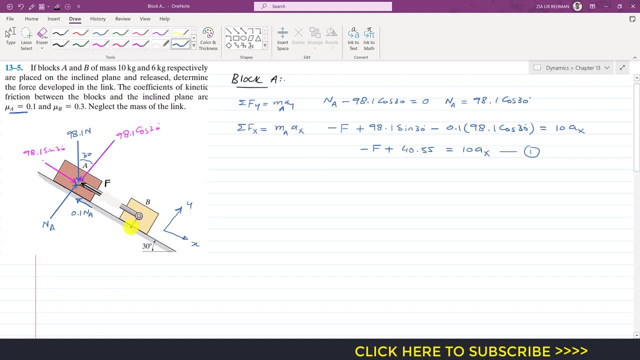 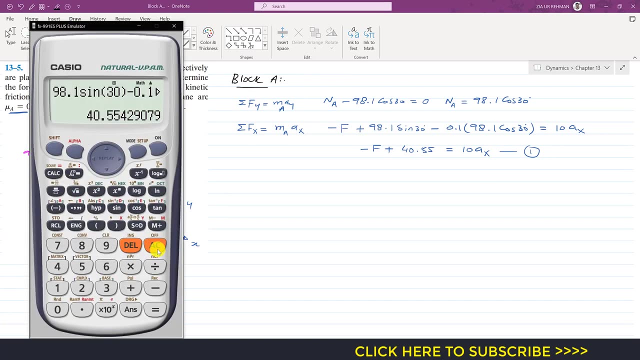 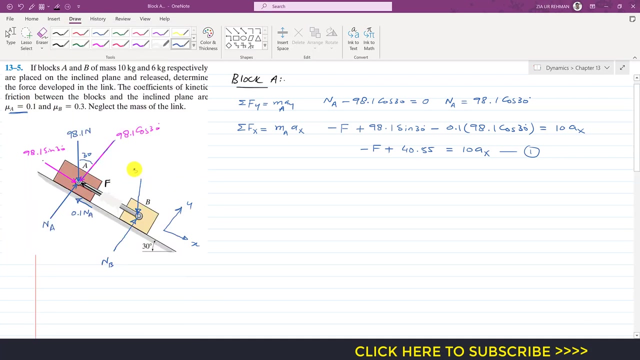 analyze this block b as well. right? so again we will have the normal force on this block b as well. let's say that is n b, right? the weight of this block b will be acting vertically downward and this will be 6 times 9.81, which is 6 times 9.81 is 58.86. so this is 58.86. 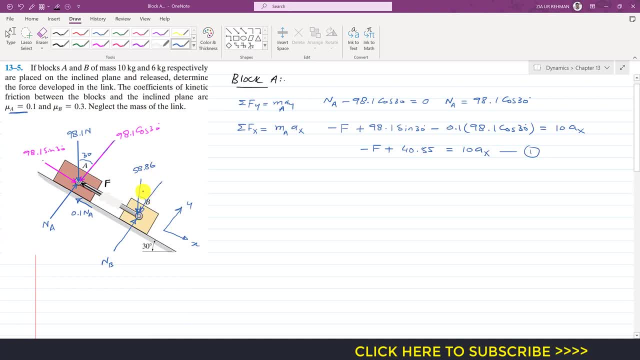 and if we resolve this into its component, so it so it will be making 30 degrees here, so this will be 58.86 cos of 30 and similarly we will have the sine component, which will be acting like this and if this block b is applying the force on this block a in this direction. so 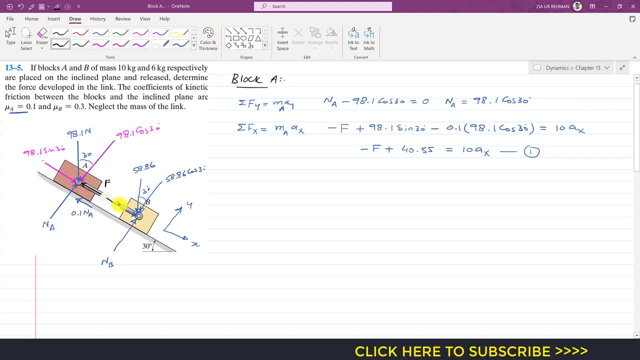 that block a will apply the force on this block b in the opposite direction. right, so we will have that same f force here as well. right so now, if i consider block b and if i apply the equation of motion, now, if i apply the summation of forces along y equals to, now. this time it will be equal to m, b, a, y and again a. y is. 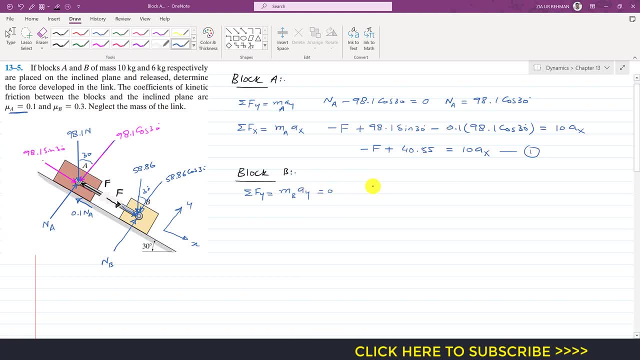 0, so this will be equal to 0, right? so now this n b is acting in the positive y direction, so i have to write n b minus this cos component, which is 58.86 cause of 30 degrees. so from this we can say that n b is. 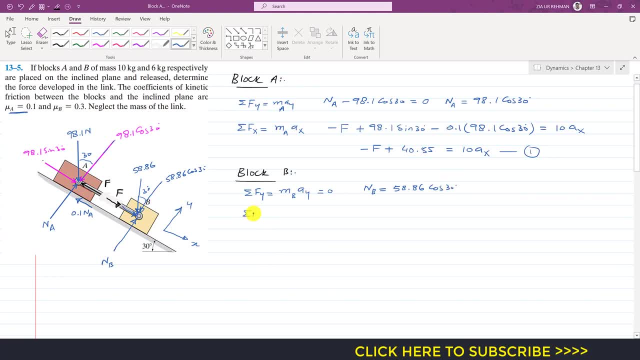 equal to the cost component of the weight. similarly, if i apply the summation of forces along x, equals to m, b, a, x, right. so now, as we can see that this f is acting in the positive x direction, so i have to direction, so i have to write plus f plus this sine component. this sine component is 58.86. 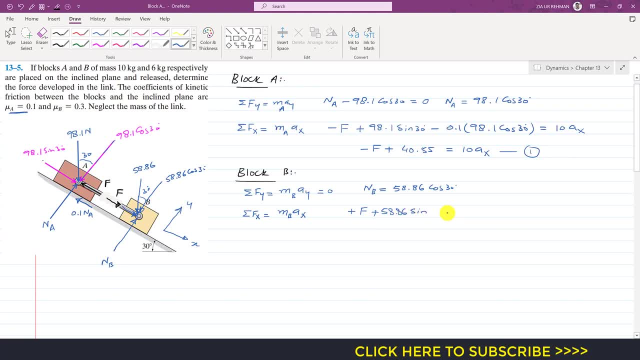 sine of 30 degrees and similarly we will have that friction force as well, right, and it is acting up the incline. and this is now this time it is 0.3 times and b. right, this is this: friction force is 0.3 times and b and it is acting in the negative x direction. so i have to write minus 0.3 and nb is: 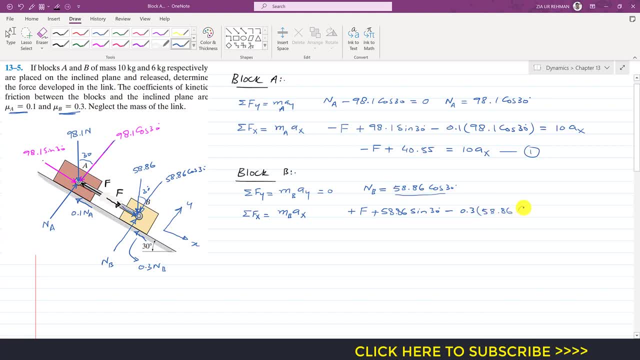 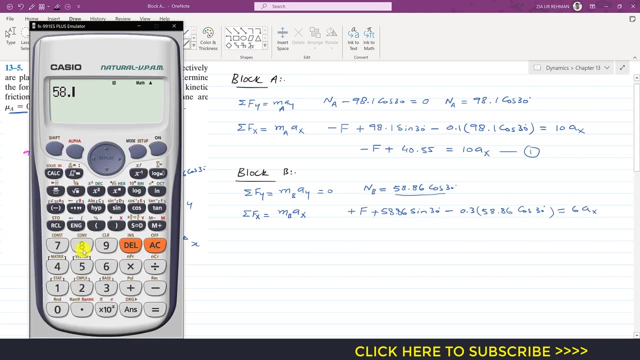 58.86 cos of 30 and this will be equal to mb, and the mass of block b is 6 kg into ax right. so now we can simplify it: it is 58.86 sine of 30 minus 0.3 into 58.86 cos of 30. 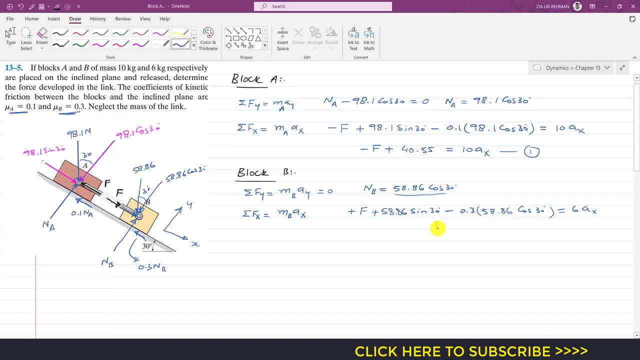 so this gives me 14.14, 14.14 and this is f plus 14.14, equals to 6 ax. this is equation 2, right? so now if i add equation 1 with equation 2, right, so this is my equation: 1 minus f plus 40.55 equals to 10 ax. so now, if we add both of these equations, 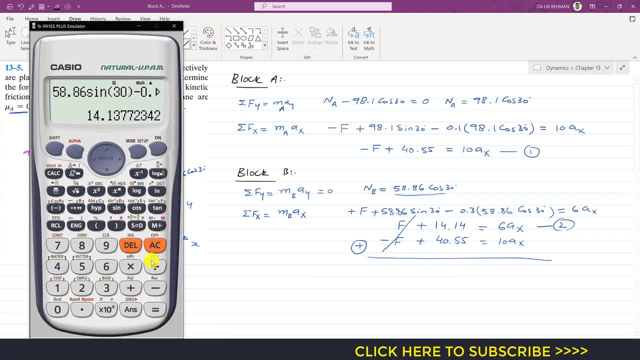 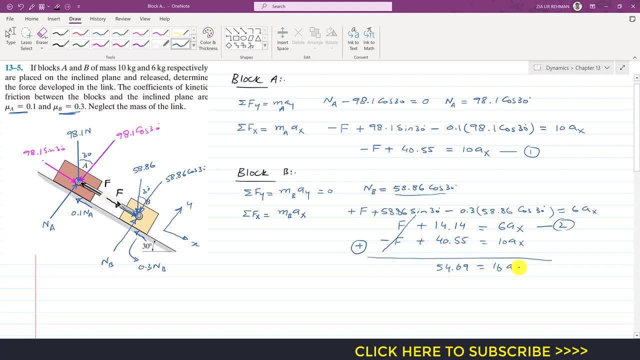 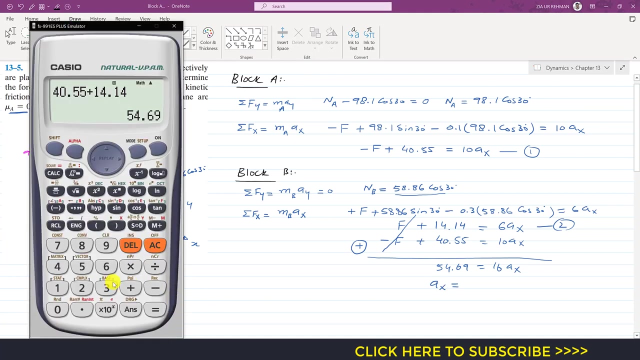 so this f will cancel out. this will be 40.55 plus 14.14. this is 54.69. this will be equal to 16.16 ax, and if we divide both sides by 16, so we will get ax. so ax is equal to 54.69 divided by 16.